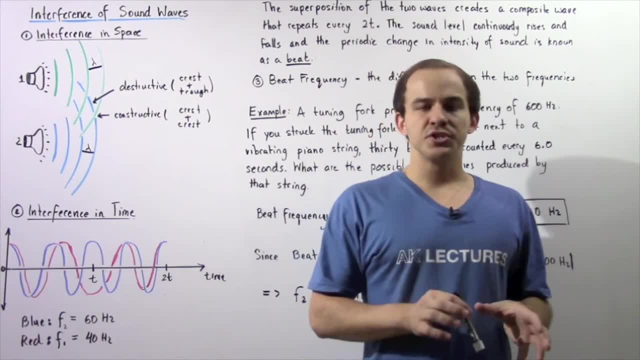 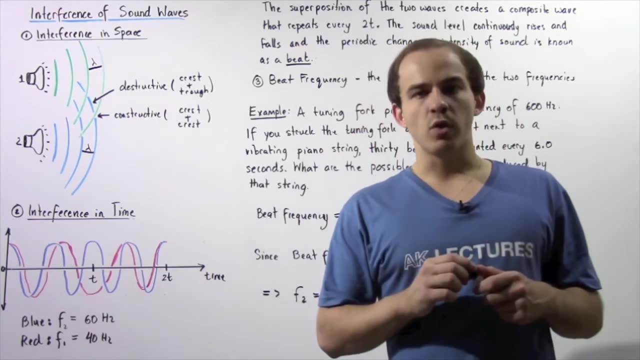 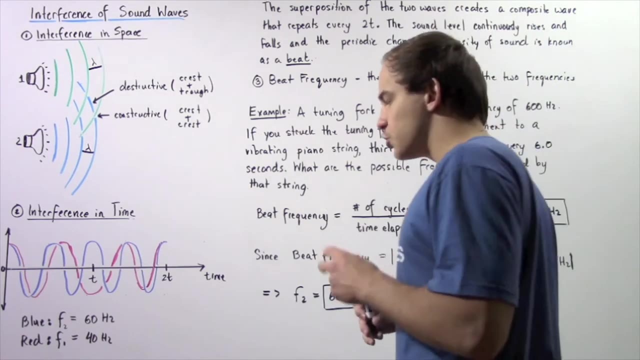 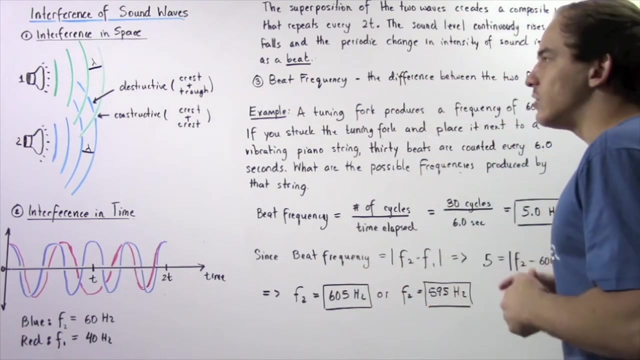 Previously we spoke about interference and superposition of waves. Now we're going to examine specifically the interference and superposition of sound waves. So let's begin with the interference of sound waves in space. Let's suppose we have two loudspeakers: loudspeaker number one and loudspeaker number two, each producing its own sound wave. So loudspeaker? 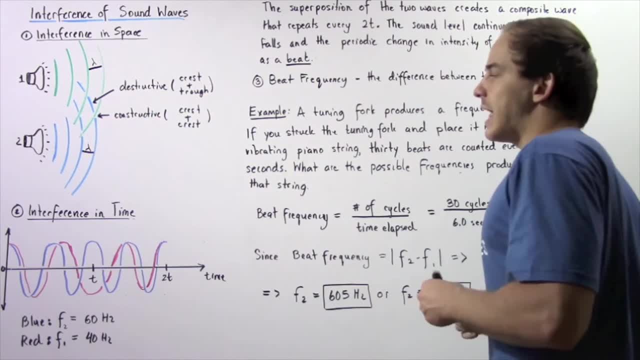 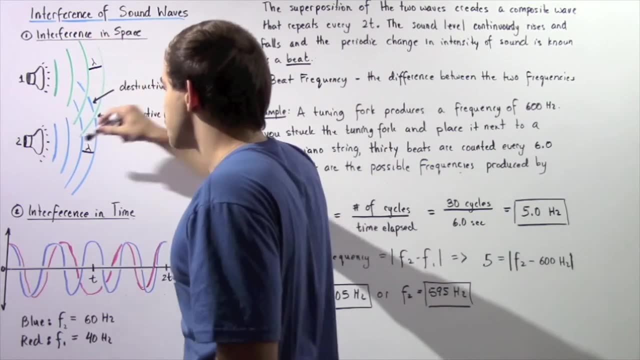 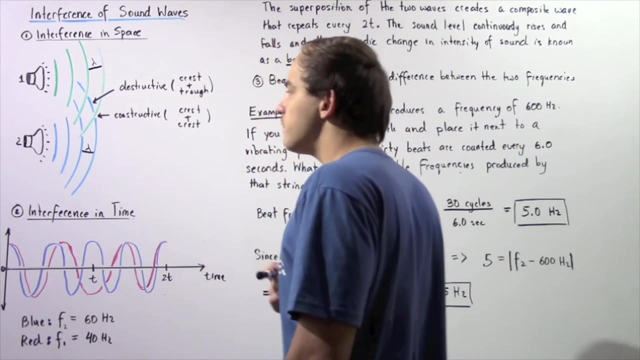 one produces the green sound waves and loudspeaker number two produces the blue sound waves. Now the green regions and the blue solid regions. solid lines are the crests. Those regions correspond to the compression regions of our air molecules And the regions in between the solid lines are: 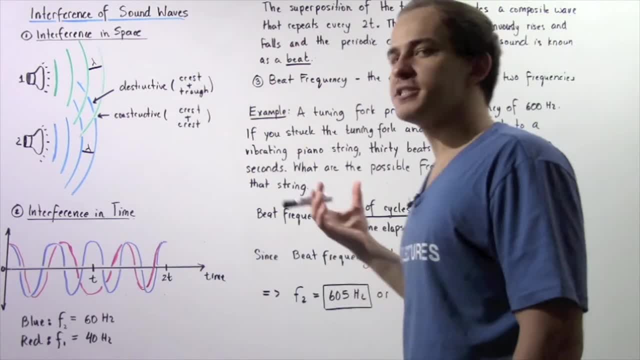 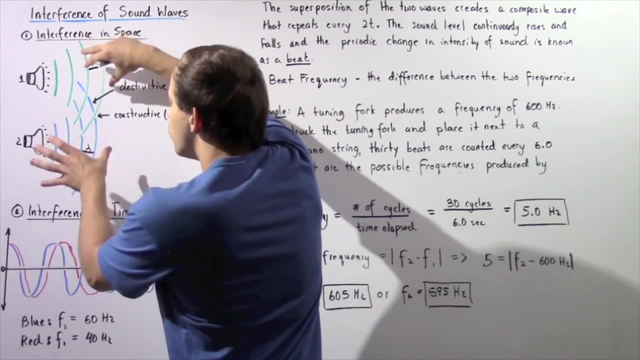 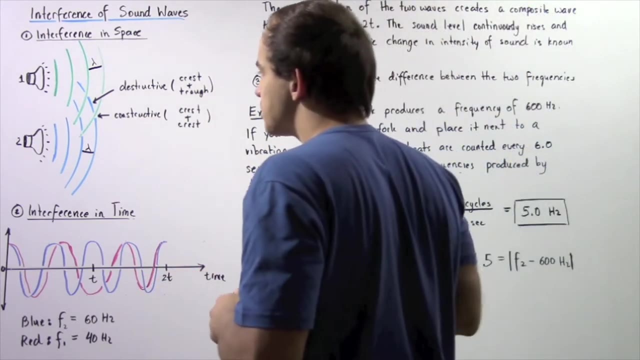 the troughs. Those correspond to the region of expansion of the air molecules. Now notice that eventually these two waves will interfere with one another, And so to create the composite wave we have to apply the principle of superposition. Now notice at the regions where 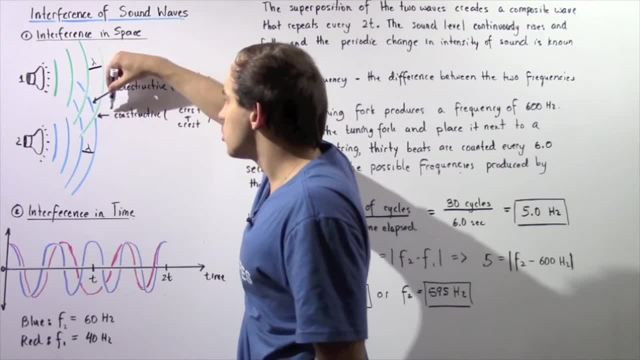 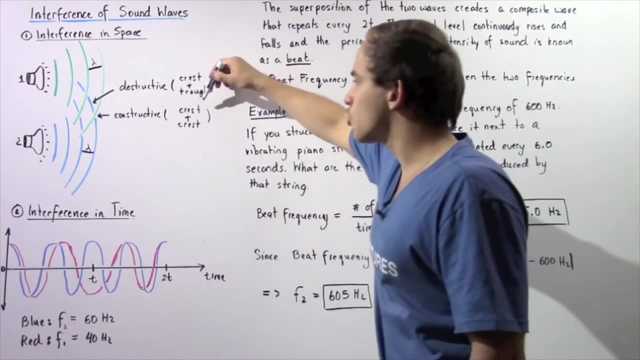 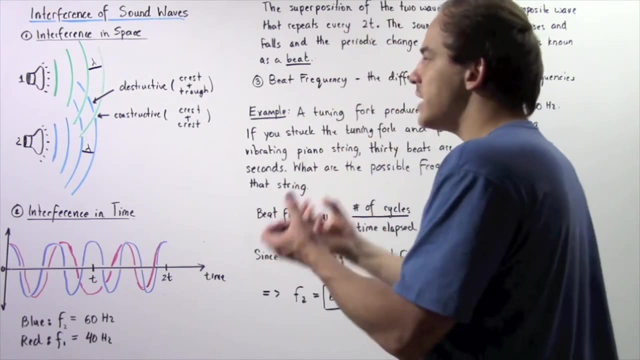 the crest, where the green crest meets the blue crest, those regions are the constructive regions, That's where constructive interference takes place. So the crests meet the crest and the amplitude becomes larger. So the amplitude of the composite wave created from the superposition of these two waves. 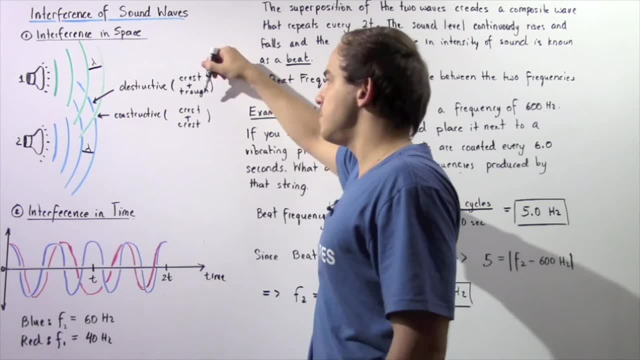 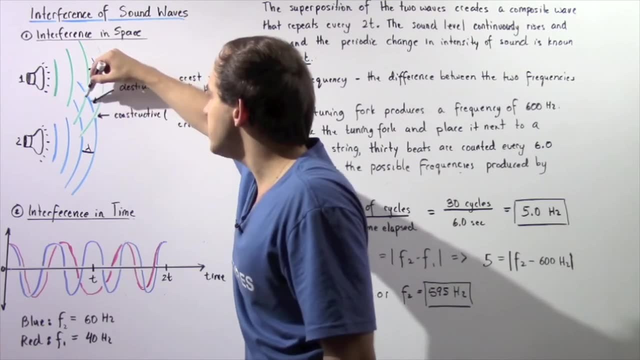 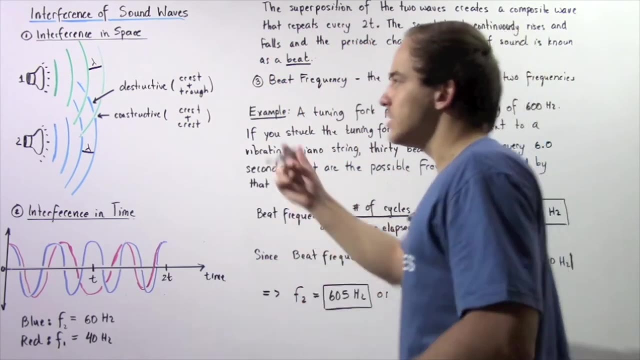 is largest at this region where the crests meet the crests. Now notice where the crests meet the trough, So where the blue crest is in between these two green crests, that's where constructive interference takes place. So our amplitude is smallest in those regions And this is known as 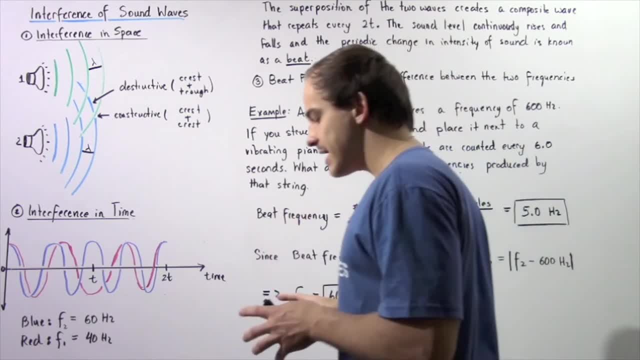 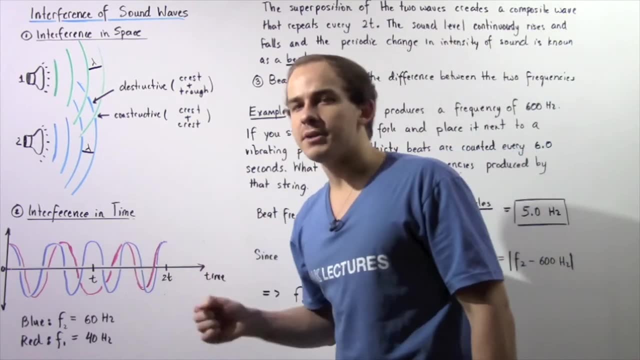 interference of our sound waves, So the amplitude of the composite wave created from the superposition of sound waves in space. Now let's move on to interference of the sound waves in time. This creates a phenomenon known as beat frequency, as we'll see in just a moment. So let's suppose we 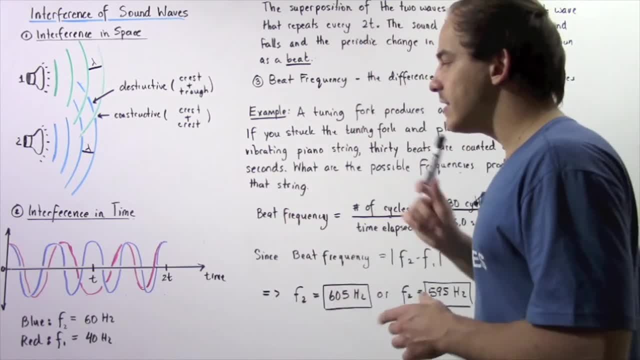 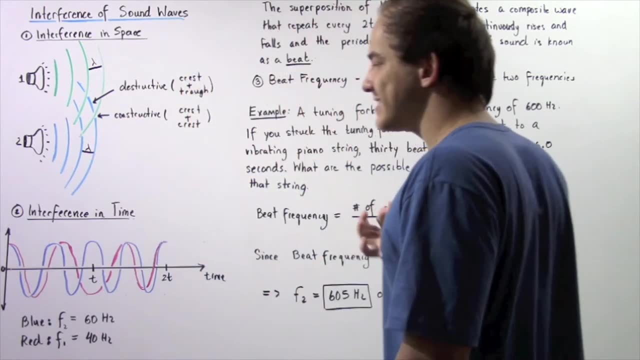 have the following two waves: The blue wave and the red wave. Let's suppose that the maximum amplitude of each one of these waves is exactly the same. Let's suppose they begin at the same exact region and the maximum amplitude of each one of these waves is exactly the same. So let's. 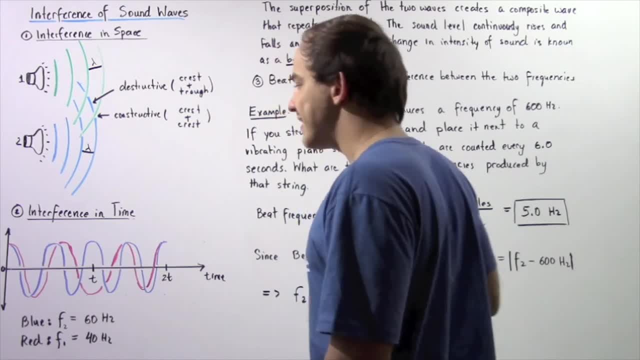 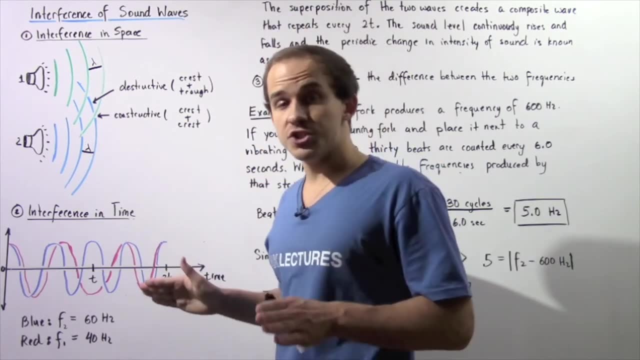 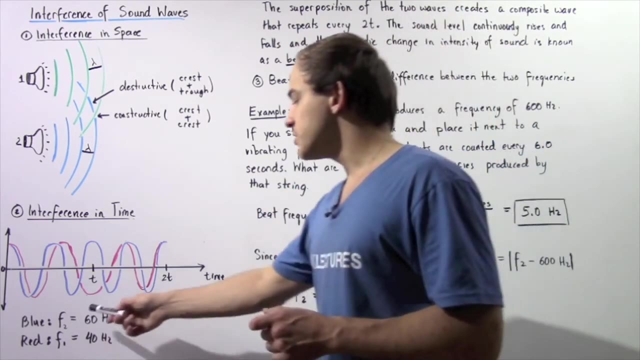 suppose that the minimum amplitude of each one of these waves is exactly the same. So let's suppose that the minimum amplitude of each one of these waves is exactly the same. So let's suppose that the minimum amplitude of each one of these waves is exactly the same. So let's suppose. 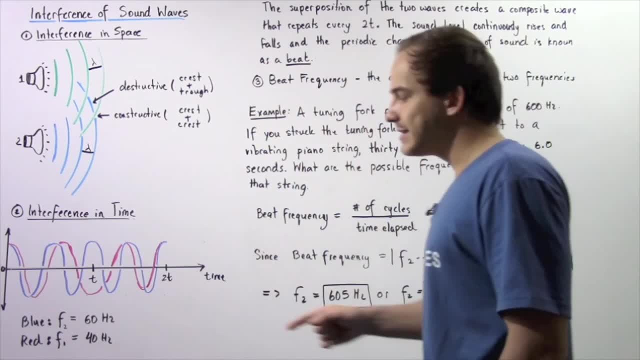 that the consumed more hearth and also the无armen inertia have a higher frequency. Meghan Subdivner would say: scientists quickly, gymnastics of which has a very important thing on. the episode is absolutely evident in this example. So let's attached: ac executed Ne eş-. 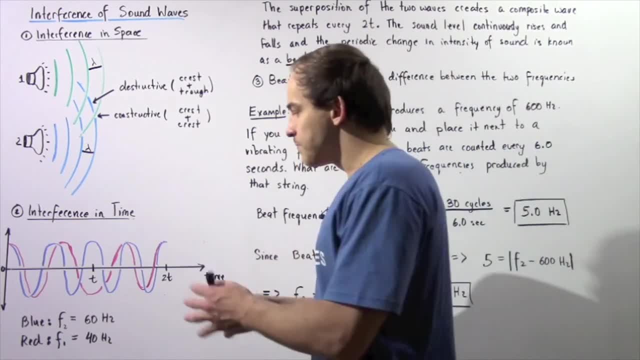 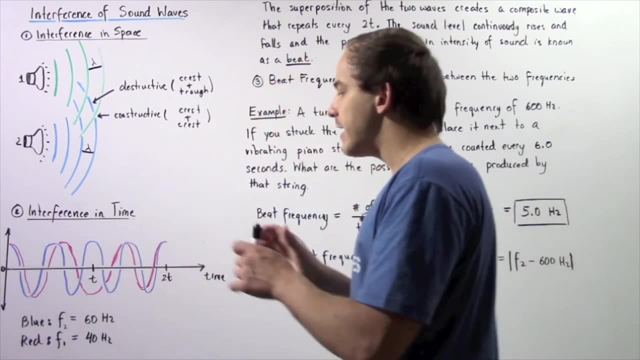 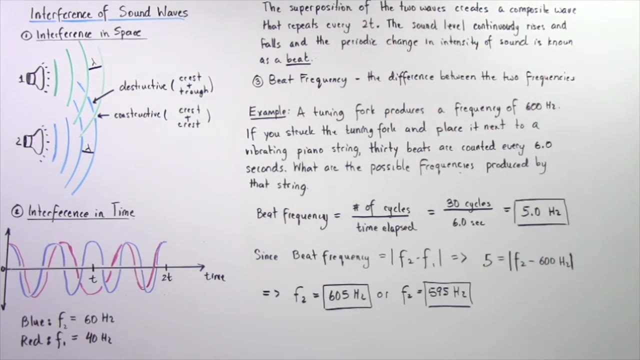 mushes компosič make the Amin. So if we examine the complex wave that is produced from the interference, from the superposition of these two waves, that wave is known as the composite wave. So the superposition of the two waves creates a composite wave that repeats itself every single 2t seconds. 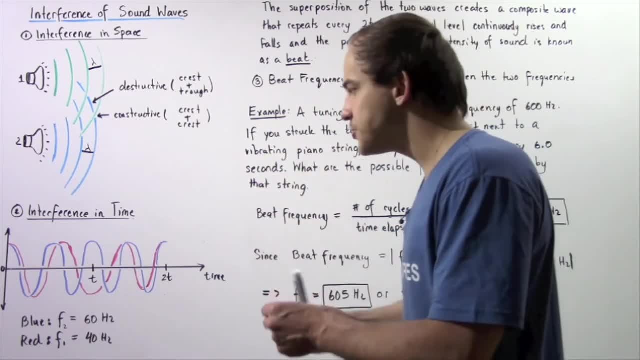 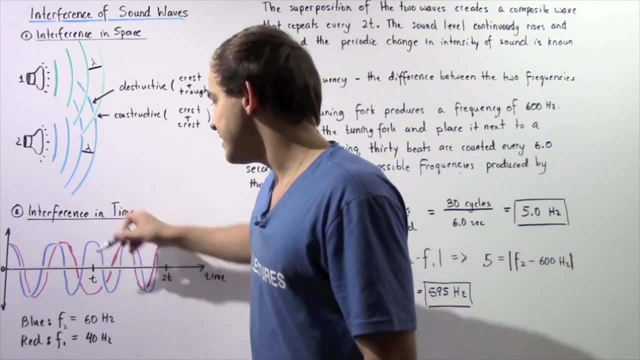 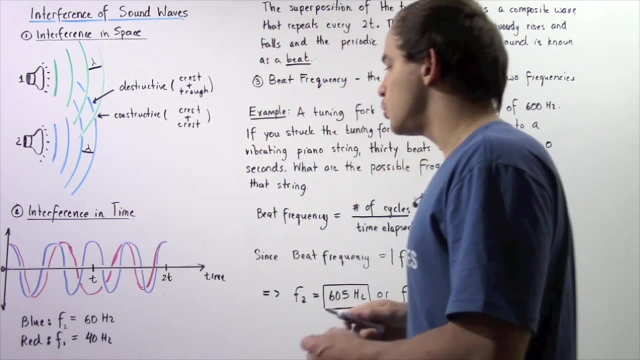 where 2t is simply the number of seconds after which the composite wave begins to repeat itself. Notice, at time equal to t, the two amplitudes cancel each other and the composite wave at this time has an amplitude of 0.. 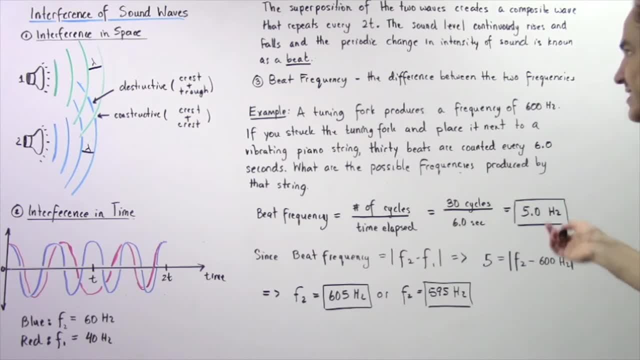 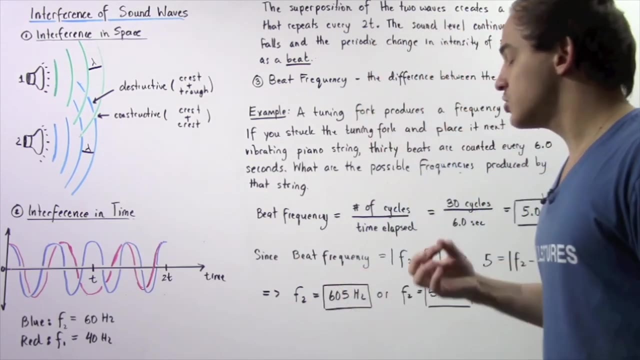 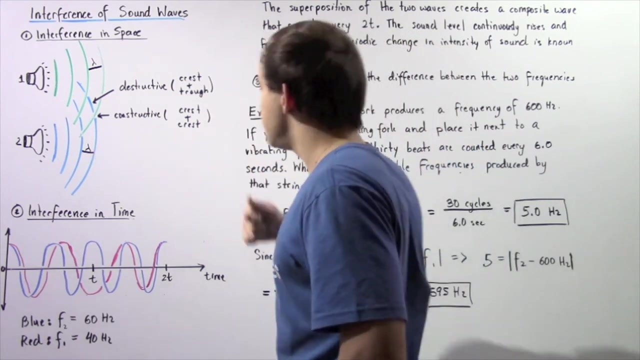 Now the sound level continuously rises and falls as our composite wave travels this way, and the period change or the periodic change in intensity of the sound is known as beats, So the beat is reduced. This is the result of the fact that there is a difference in frequency between wave number 1 and wave number 2,. 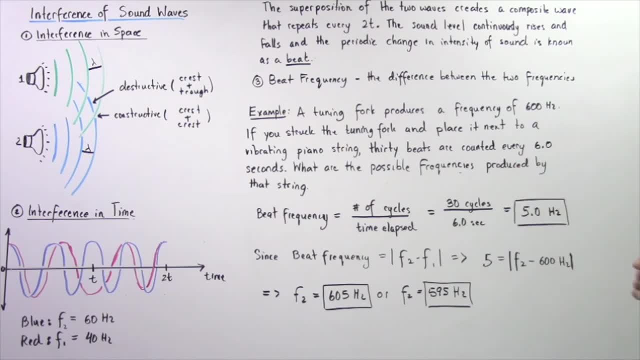 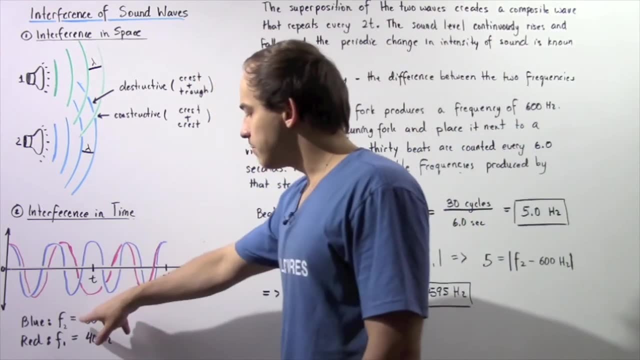 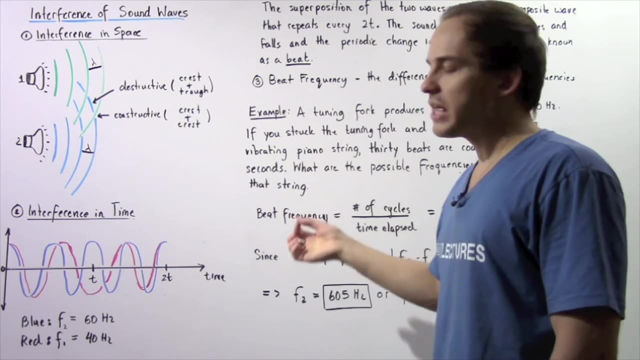 and we define something known as the beat frequency as the difference between the two frequencies of our two waves. So, for example, in this case the beat frequency is simply the absolute value of 60 minus 40, so that's 20 hertz. 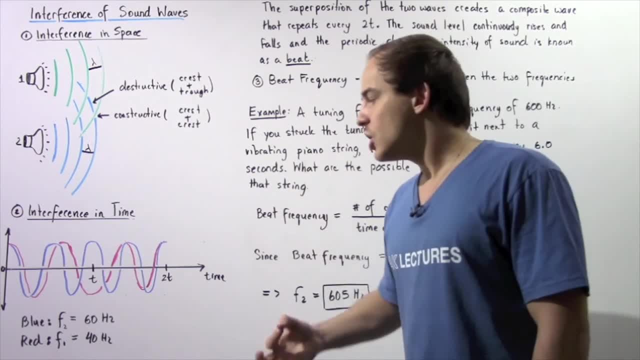